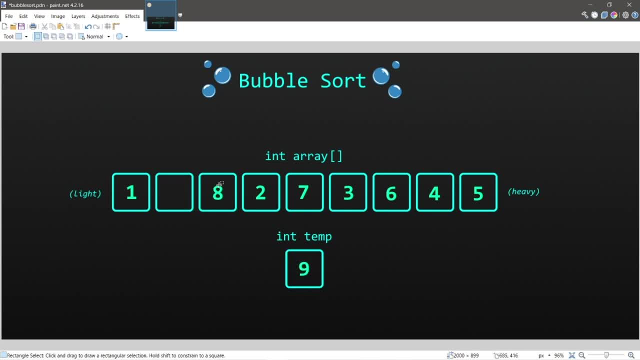 will move our first element into temp, Move the second element to where element one was and then move temp to where element two is, and then we would just repeat this process. So we will lap through this array once for each element that is available. So let's just speed up the footage here and I will show you manually a bubble sort. 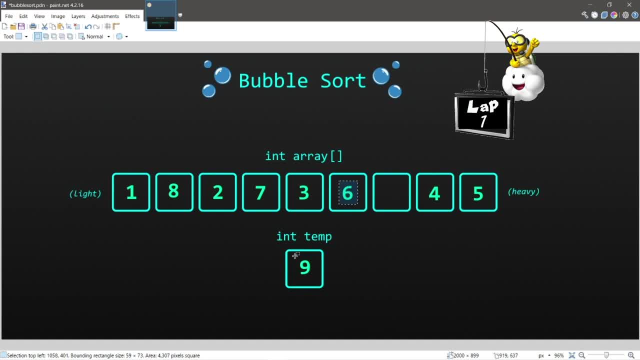 So let's just speed up the footage here and I will show you manually a bubble sort. So let's just speed up the footage here and I will show you manually a bubble sort. As you may have noticed, the bubble sort algorithm really isn't that efficient. 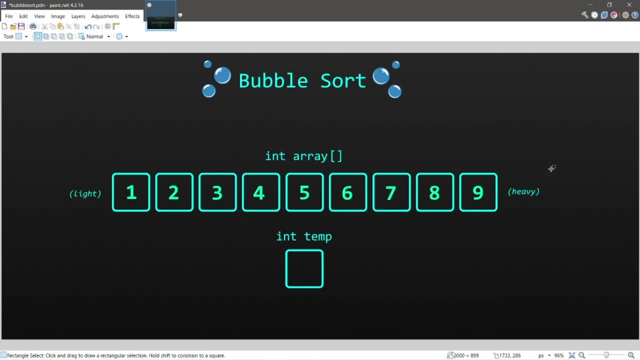 even when working with smaller data sets. In most real world applications you'll probably use a different sorting algorithm, but this is still a good thing to learn. So the bubble sort algorithm has a runtime complexity of O of n. squared. It runs in quadratic time. 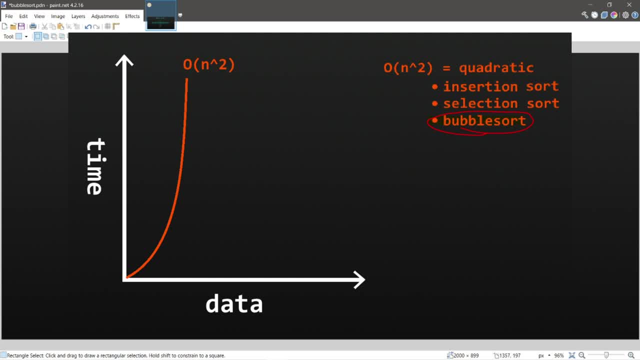 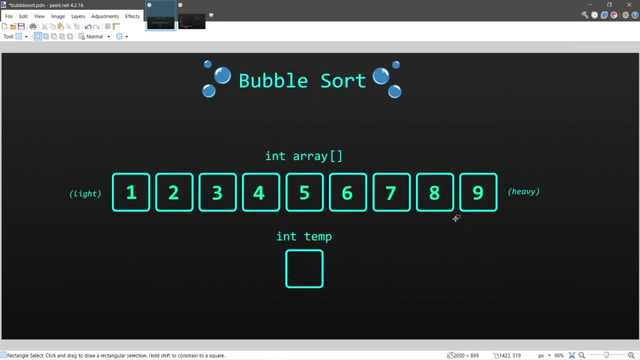 So the larger the data set, the more and more inefficient that this sorting algorithm is going to be. With a small data set, it's not horrible, but there's definitely better algorithms out there. So for practice, let's create our own bubble sort algorithm. 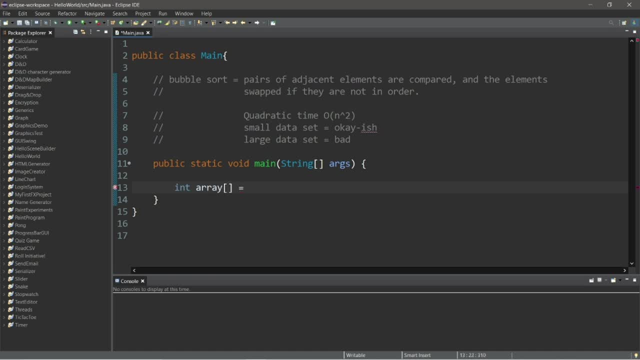 Alright, let's create an array of integers. Alright, let's create an array of integers. Alright, let's create an array of integers And assign some random numbers. Make sure that they're not in order, because, well then, that would defeat the purpose of this program. 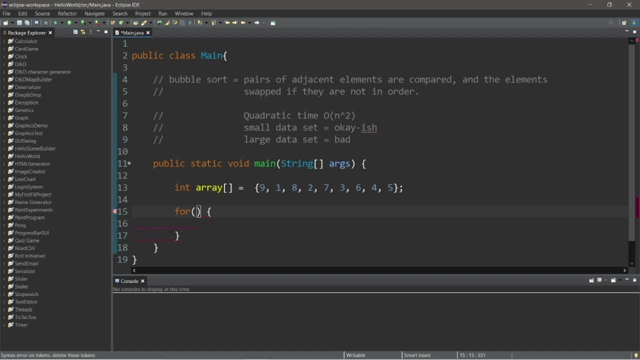 So at the end we'll just display all the elements of this array using an enhanced for loop. For i in array we will display with a print statement, not print line, whatever i is during each iteration. So let's just test this. So I have all the elements in. 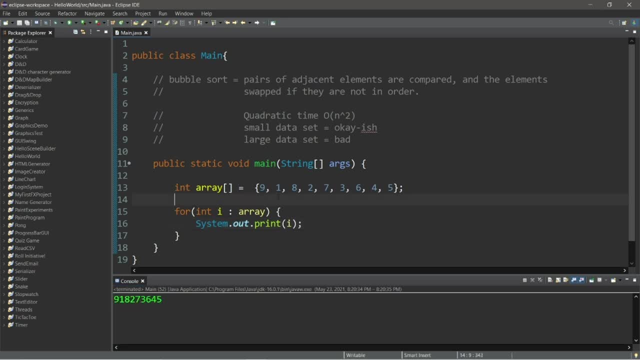 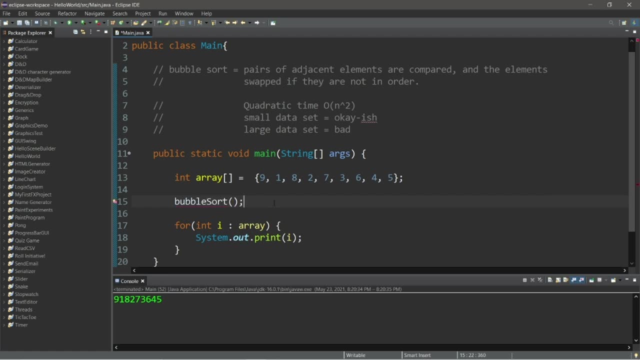 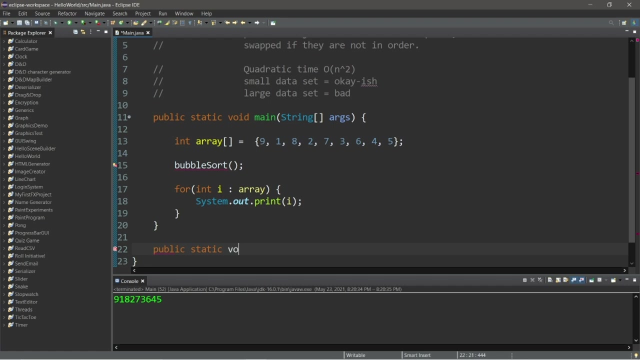 my array printed and they're currently not in order. So we'll need to declare a bubble sort method- Bubble sort, And then we will need to define this outside of our main method. So: public static void- we're not returning anything. Bubble sort, And then we will need. 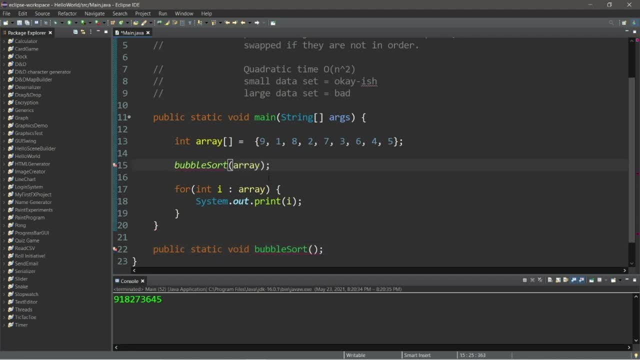 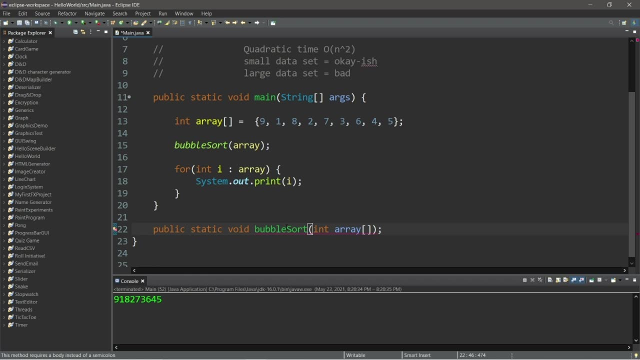 to pass in an array. So that will be the argument array And we will accept int array. Okay, so this is actually really easy to do, So let's go ahead and create an array of integers. Alright, so let's go ahead and create an array of integers. Alright, so this is actually really easy to write. 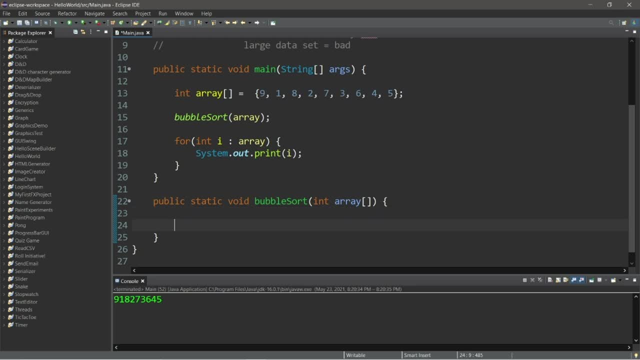 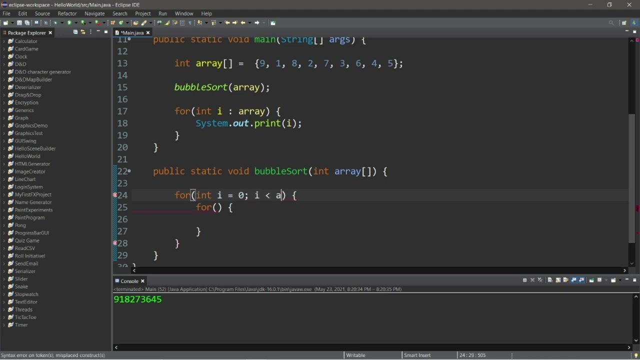 even though the bubble sort algorithm really isn't too efficient. So I guess that's one benefit. So we'll need nested for loops And then the outer for loop will be int. i equals zero, i is less than array dot length minus one. i plus plus. And let's do the same thing with the. 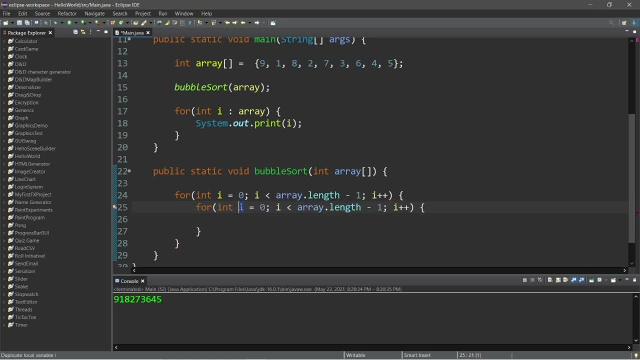 inner for loop. But we can copy what we have. So let's go ahead and create an array of integers. What we have change i to j And this is going to be array length minus i minus one. So we're going to check to see if array 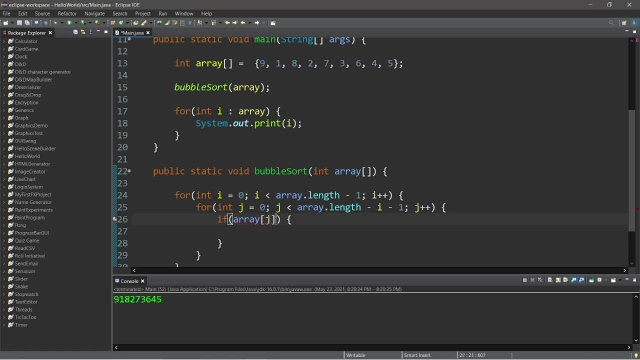 at index of j is greater than that will be for ascending order, is greater than array at index of j plus one. So that would be the next adjacent element. So if this number is greater than this one, we should switch these two elements around And we'll need the assistance of a temporary. 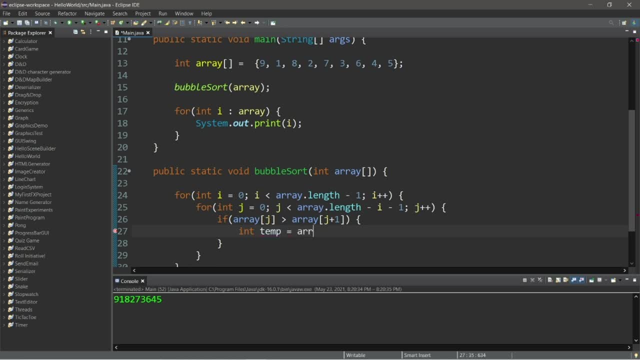 variable. So let's declare int temp equals array at index of j, Then we will take array at index of j, set this equal to array at index of j plus one, And then, lastly, we have array at index of j plus one equals whatever stored within temp. And honestly, 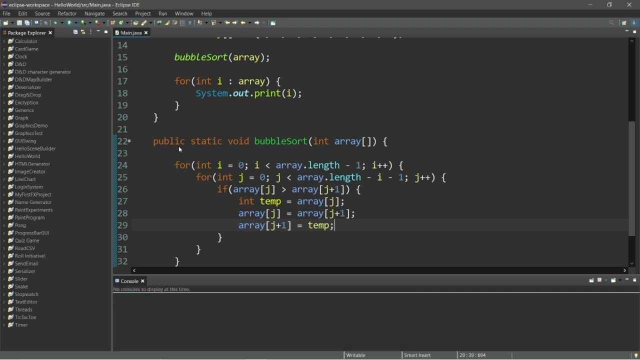 that's all there is to it. So this should sort our array, And it's in ascending order. So if you need this in descending order, we would just swap this greater than sign with a less than sign, And now this is in descending order. So, even though the bubble sort algorithm really isn't,